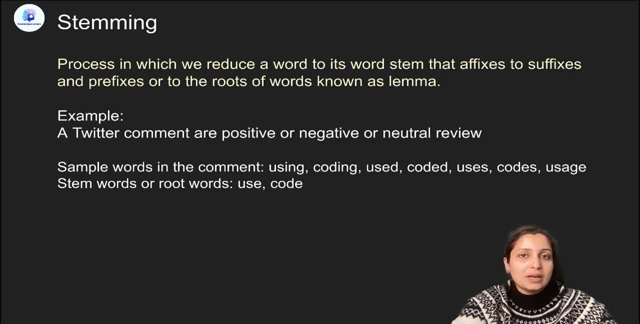 But we will first explore stemming hands-on to get more acquainted with different kind of stemming used. What is the advantage of one kind of stemming over another? And post that when we compare it with lemmatization. So let us get hands-on with stemming. Please open your Jupyter notebooks along. 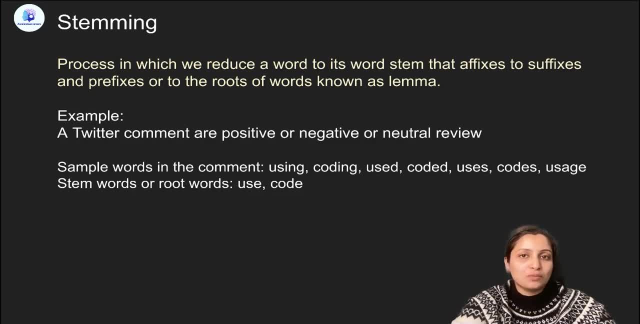 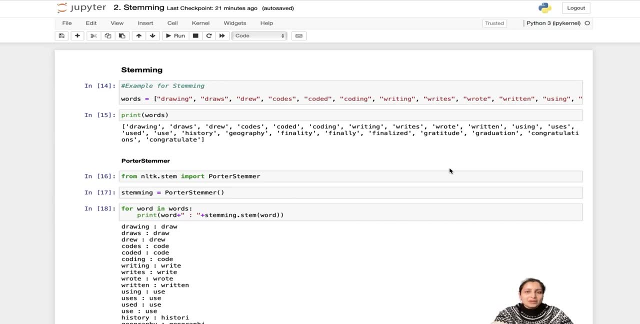 with me and follow the steps alongside. I will share the Jupyter notebook GitHub link here in the video. You can use that as well. So now let us implement stemming hands-on. I hope you have your Jupyter notebooks opened, So we will start with a new notebook here just for stemming And 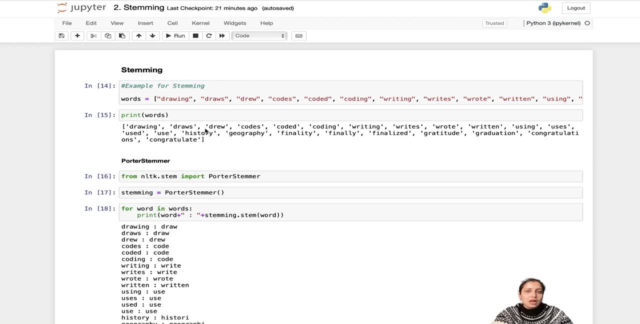 we look at different kind of stemming, So let us start with a new notebook here just for stemming. What are the advantages? How do they work? What are the disadvantages? Which one is better? Whether stemming is better or lemmatization is better, So we will go with that. Let us take a set of 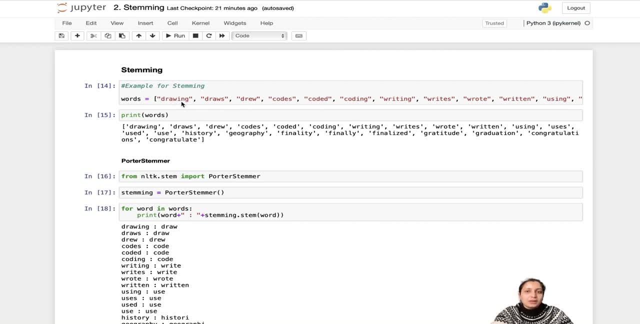 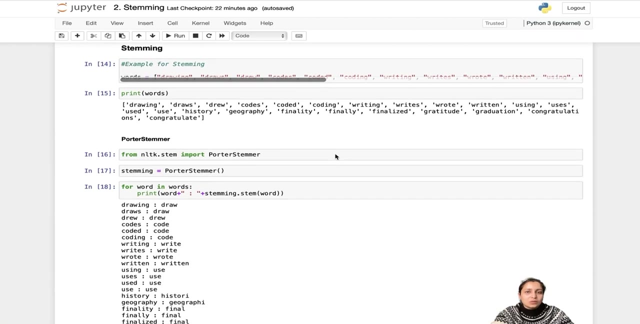 words here. So the set of words which I have taken are drawing, draws, drew, codes, coded, coding, writing, writes, wrote, written, using, uses and so on. So you can see those words here just in the below cell. I have printed those words. 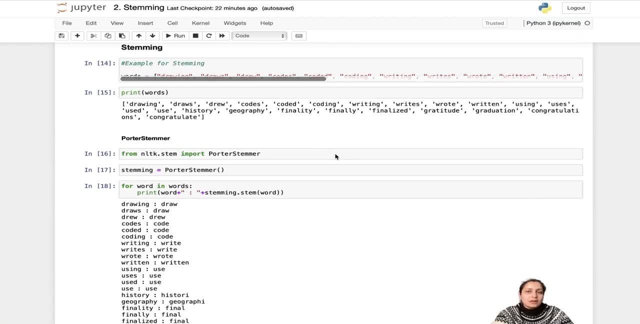 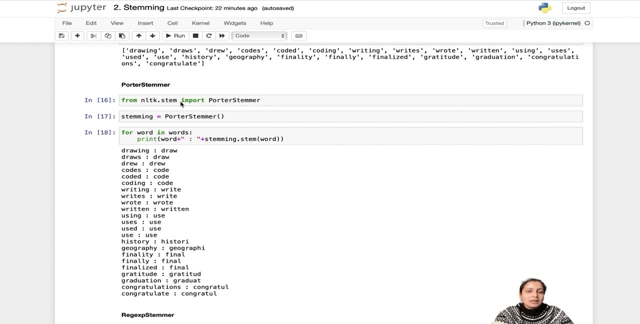 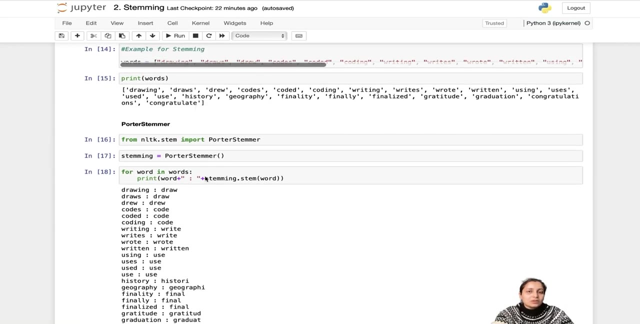 I have taken all these words. Now let us try out the first kind of stemming, which is Porter Stemmer. So in Porter Stemmer you can just import it from nltkstem and then instantiate the object. Once you have instantiated, we will be running a for loop across the words list so that 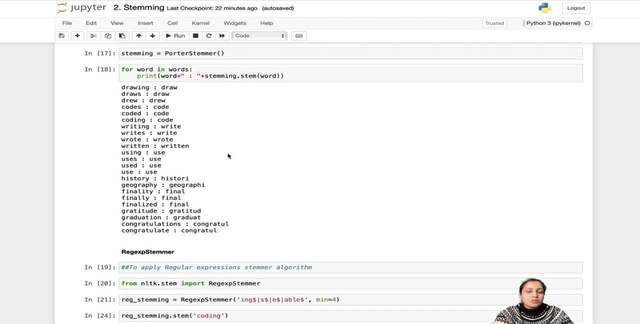 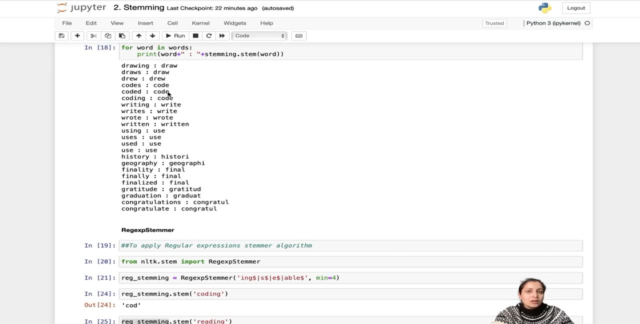 each word is stemmed And we will be printing the stemmed word alongside the word in this format, as shown here. So if you could see that for some words it is doing a great job- Like for drawing, it is doing a great job. So if you could see that for some words it is doing a great job. 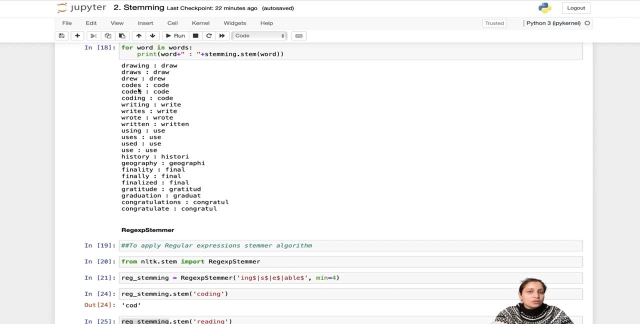 It shortens it to draw, which makes sense. For codes to code, for coding to code, writes to write. But do you see that? for wrote, it keeps wrote as such, Written, it keeps it written as such. For using, uses, used, everything it has been shortened to use. But if you see it, 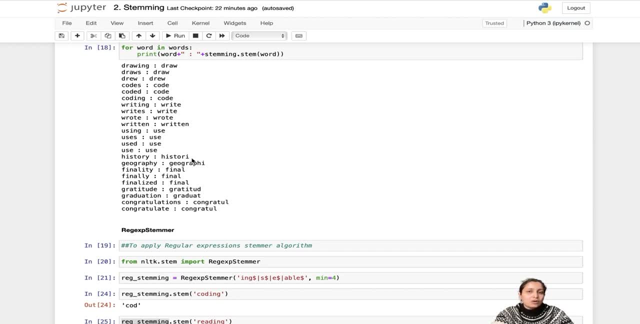 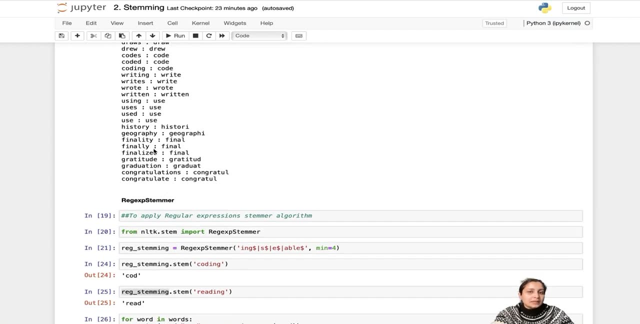 does a very bad job for history. it just changes it to a meaningless word history, Geography- again a meaningless word there For finality: finally finalized everything. it reduces to final Again. if you see another word: graduation. 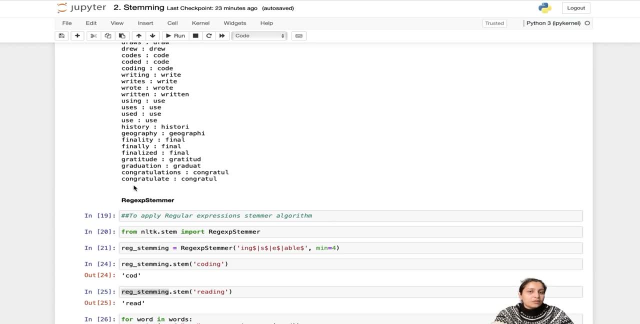 it generates a meaningless word graduate. And for congratulations, it generates a meaningless word called congratul. So even though it reduces the word to its root or to its stem, it doesn't always generate the meaningful word. Now let's look at another kind of stemming. 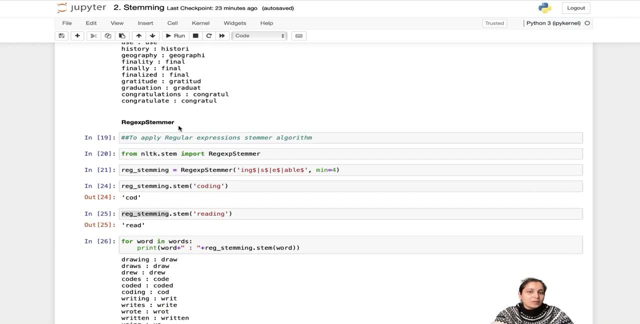 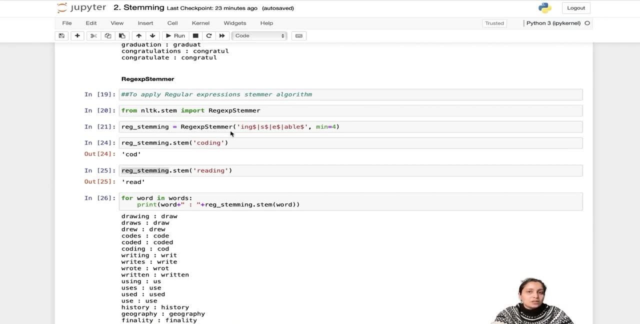 which is regular expression: stemmer, regex, stemmer. imported from the nltkstem And instantiated When you are instantiating it. if you just instantiate it without any parameters, you will get an error. So you have to provide the regular expression there and minimum length. 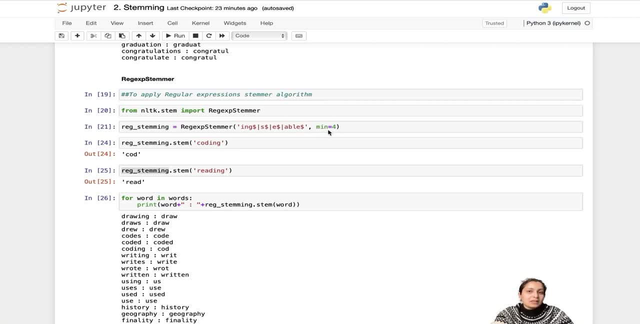 The minimum length means it will only stem if the minimum length is 4 or whatever you provide And the regular expression. what it means is ing. dollar means if in the end of the word it's ing S. dollar means if in the end of the word it's s, then it stems E dollar means if in the end 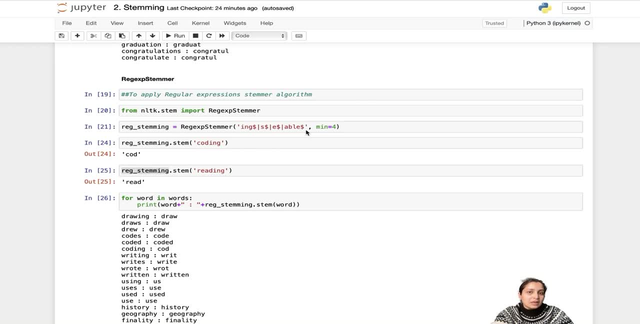 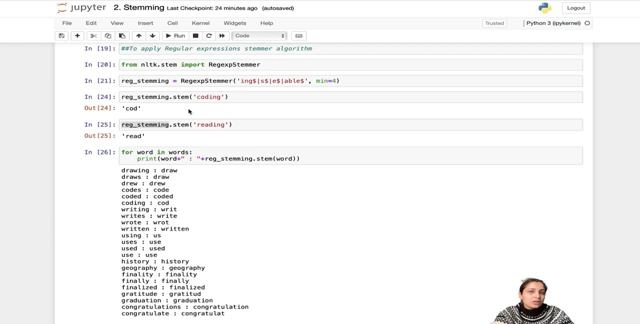 it's e. Able dollar means if there is able in the end. So let's look at some examples here. So regular stemming does stem and use stem coding. So it stems coding to code, even though it is a meaningless word, but you can customize it for reading: It stems to read. 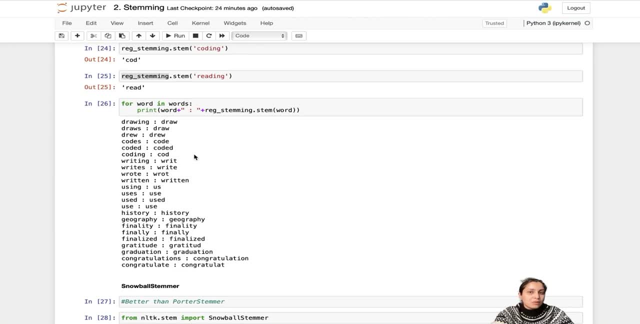 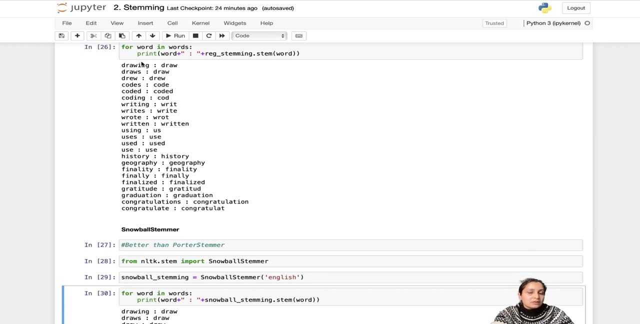 So we'll run the same loop on words list before, like before, and see how it is different from porter stemmer. So, like porter stemmer, it does successfully for drawing, draws, drew coding, coded codes, etc. The change which I see is for wrote. it shortens it as well to a. 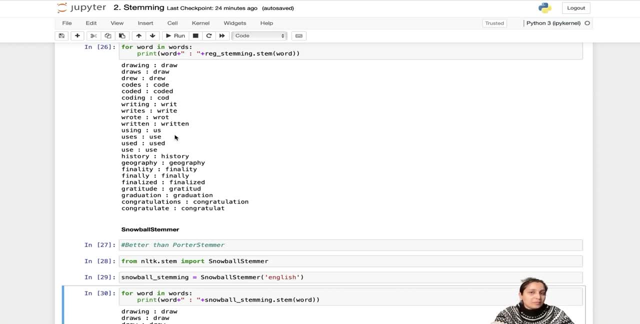 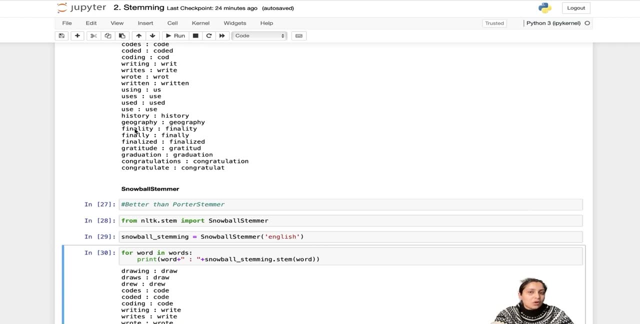 meaningless word For using, uses it shortens them. For used it doesn't shorten. And if you see the places where porter stemmer was failing, like history, geography, finality, finally, it is doing a great job here. If you see, for graduation and congratulations, it is doing a. 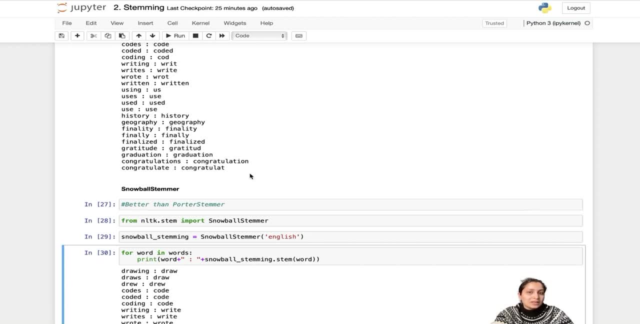 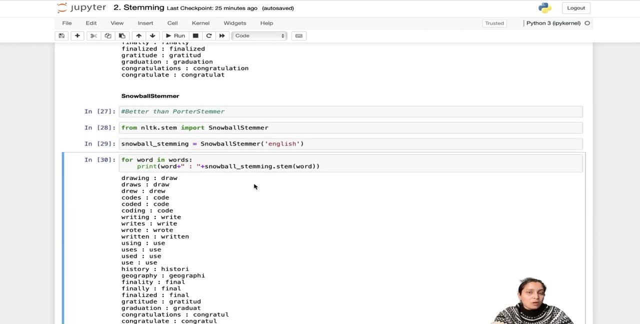 good job. It is reducing them to a meaningful word rather than a meaningless word, As it was doing in porter stemmer. Now let us look at a better stemmer class, which is snowball stemmer. It is better than porter stemmer. Let's see how. So when you instantiate snowball, 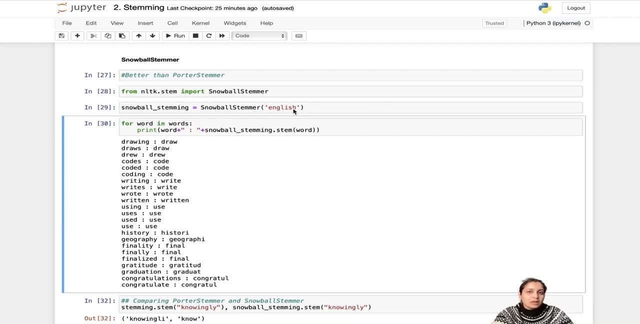 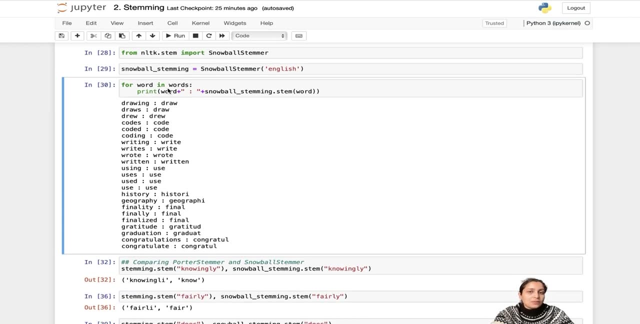 stemmer, you need to provide the language you want to stem in. So you could choose Arabic, Hindi, Sanskrit, any language. But right now we are choosing English And again we run the for loop for the words and see what's the difference. If you see, it is still doing a bad job for history. 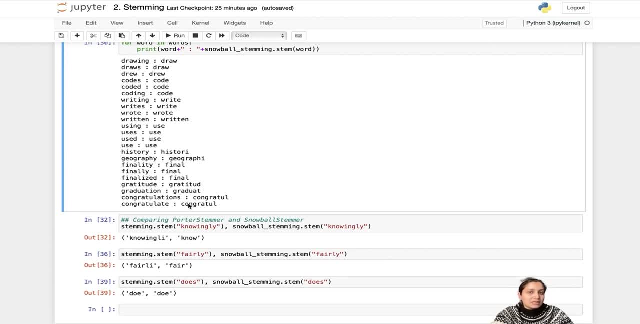 geography, gratitude, congratulations, similar as porter stemmer. then how it is different. How So for these particular list of words, it is performing almost equal to porter stemmer. So then, why did I say that it's better? So let's look at some other examples. 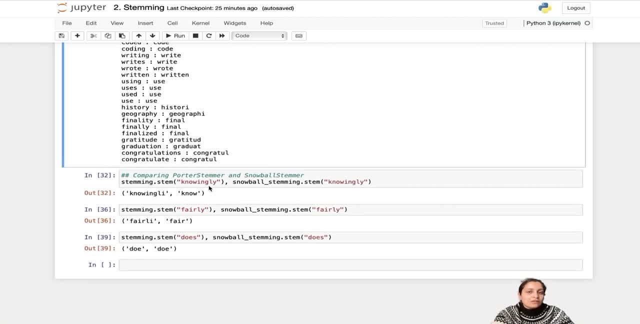 Say, suppose we have a word called knowingly And for that if we call porter stemmer it generates the meaningless word knowingly here, But if we call snowball stemmer it generates some meaningful stem called no. Similarly for another word, fairly, the porter stemmer does a bad job generating fairly here, Whereas snowball. 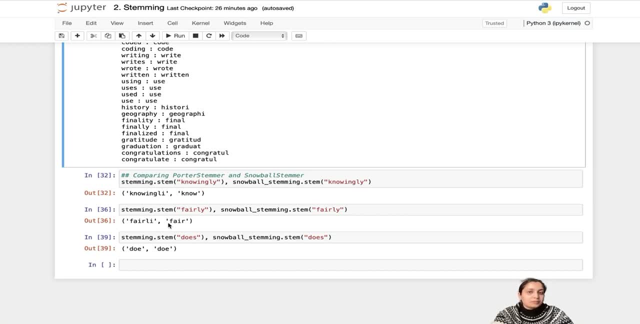 stemmer generates a correct stem, which is fair. Now let us look at an example where both of them fail. For example, does For does. if you apply porter stemmer, it generates do, And if you apply snowball stemmer, it generates do again, which is meaningless word, right? So for such cases, 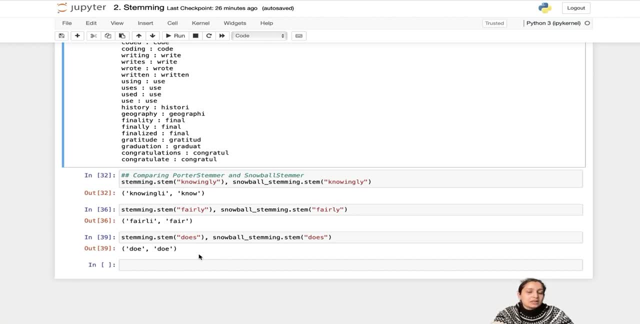 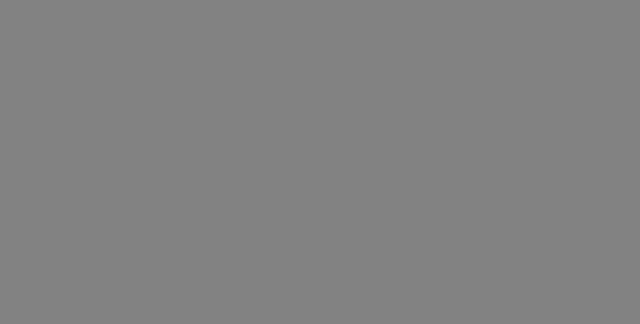 you would like to use lemmatization, Because lemmatization has a complete vocabulary within and it doesn't reduce the word to its root word, which does not have a meaning. It reduces to a meaningful root word. So we'll move towards. 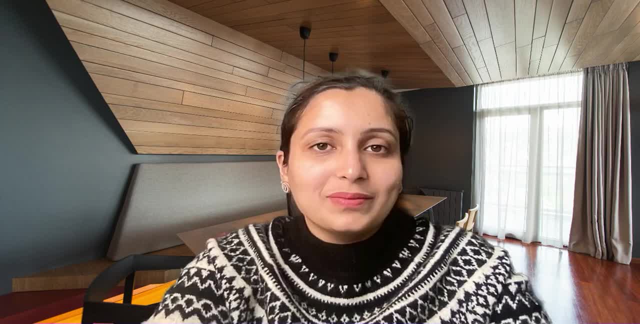 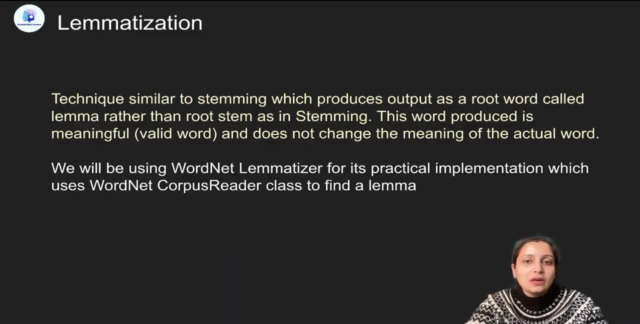 lemmatization next. So far we have looked into stemming and its hands-on applications as well some of its drawbacks. Now let us look at the next text-free processing technique, which is lemmatization. It is quite similar to stemming, but it overcomes some of its drawbacks. 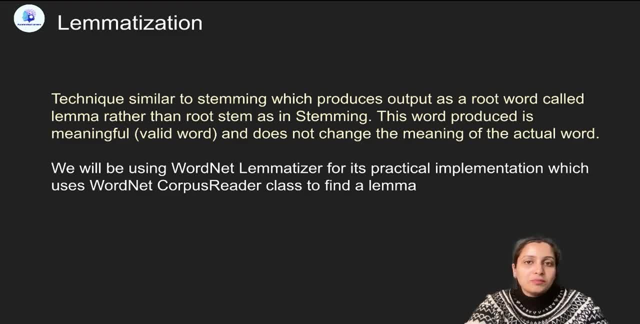 here. So, right in stemming, it produces the root word called stem, which might make sense sometimes, which might not make sense sometimes, Whereas lemmatization reduces the actual word to a root word called lemma, which always makes sense, It is always meaningful, It's a valid word. 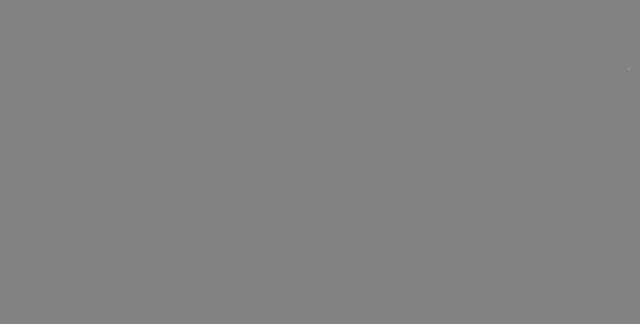 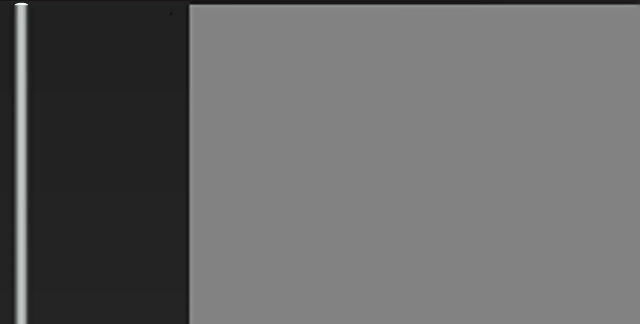 and it does not change the meaning of the actual word. We will be using WordNet lemmatizer for its practical implementation here, which uses WordNet corpus reader class to find the lemma. So let's open our Jupyter Notebook. Let's open our Jupyter Notebook. So let's open our Jupyter Notebook. 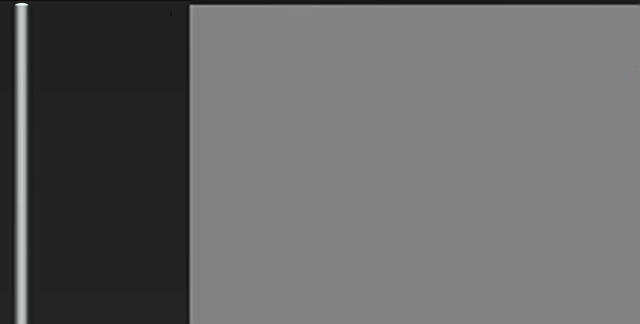 So let's open our Jupyter Notebook. Let's open our Jupyter Notebook. Let's open our Jupyter Notebook here and do hands-on learning for lemmatization. So let's do hands-on learning for lemmatization. 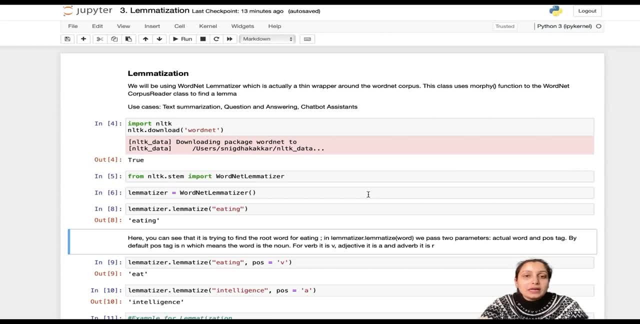 We'll be using WordNet lemmatization here, The WordNet lemmatizer, which is actually a thin wrapper around the WordNet corpus. it uses a class morphe function to the WordNet corpus reader class to find the lemma. Some of the interesting use cases for lemmatization are: text summarization: 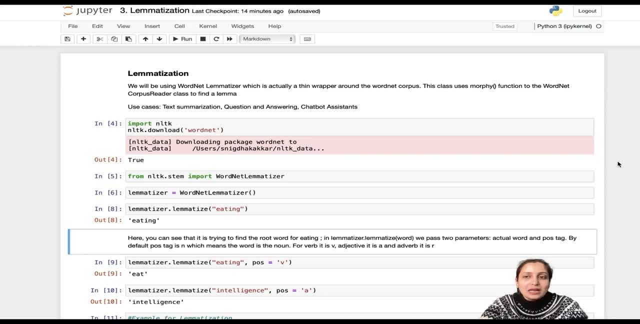 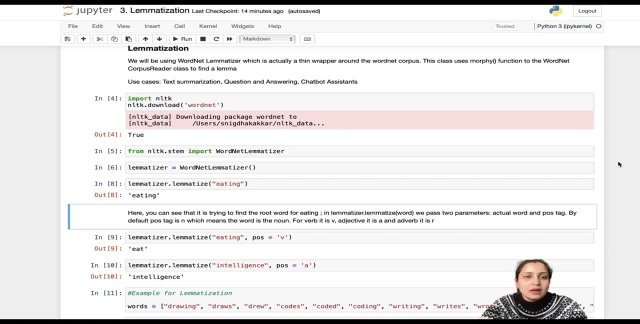 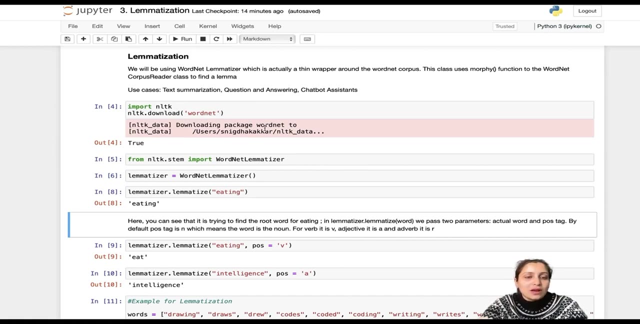 question and answering and chatbot assistant. So let's see how it's done. So some of you might face certain errors while importing WordNet lemmatizer. For that you need to import NLTK and download WordNet. Sometimes it doesn't come with the package, So once you have run this cell it will. 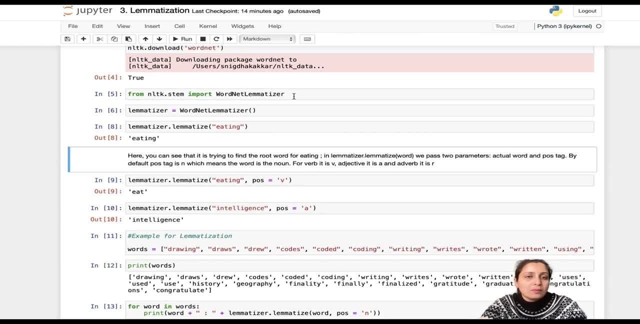 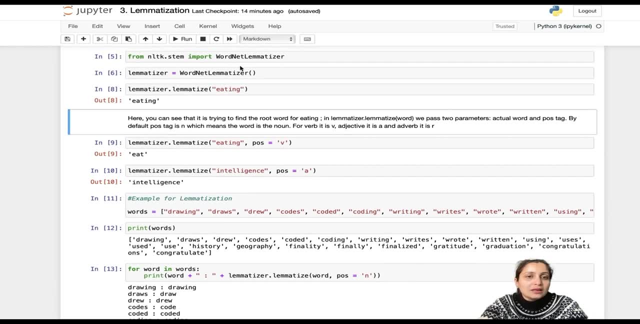 be error-free, Then you can import WordNet lemmatizer from nltkstem Then instantiate the WordNet lemmatizer object. Once you have instantiized that, then you can pass on the word of your choice. If you see that when I pass eating word here, it actually produces eating. 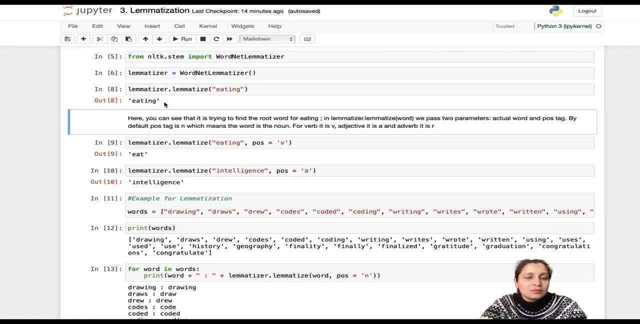 only as a result. So you would say that's a bad result it has given, because it should be eat like it was there with the stemming Underneath. there are two parameters which are entered in lemmatizerlemmatize. One of them is the actual word for which you want to produce the lemma. 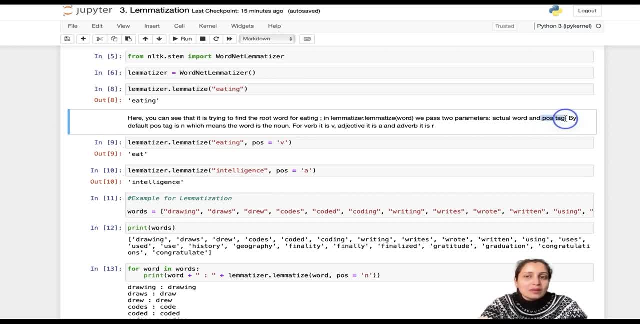 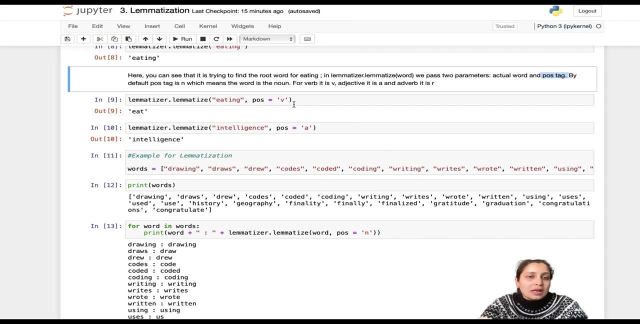 The other is the pause tag. That pause tag by default is N, which is a noun. There are other kinds of pause tags as well: V for verb adjective and R for adverb. So let's look into it. Say, suppose I give pause tag as v, In that case the lemmatizerlemmatize. 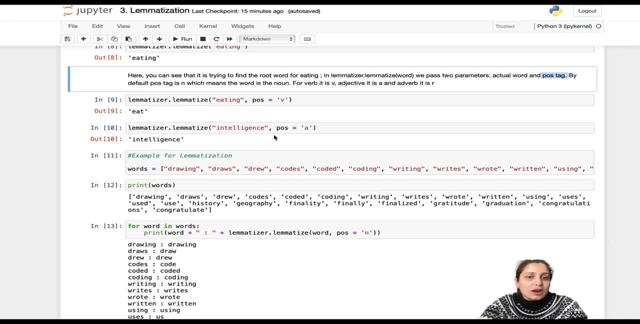 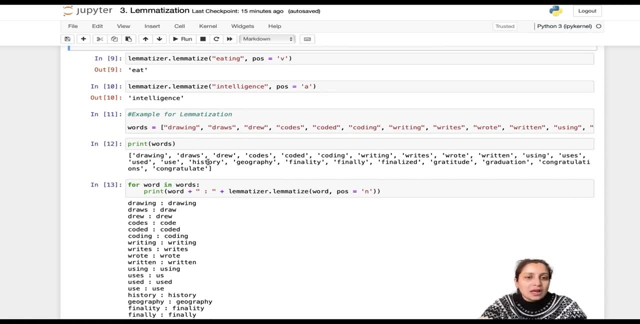 generates eat, which is correct. Same way we can try for different words. Let's take the same list of words which was there for stemming- I have printed it here so that you can see which all words I have taken- And let's try it by default by noun. So if I give pause tag as noun here, then 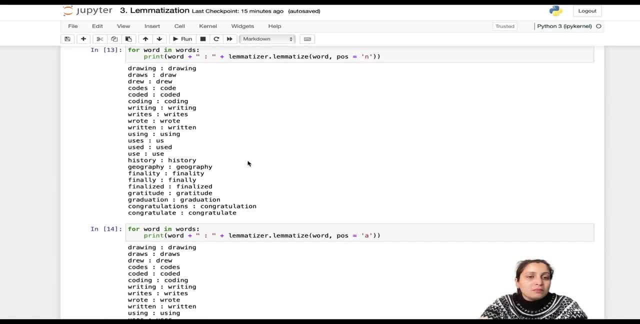 you can see the results are almost similar to stemming, but it is corrected here for history, geography and alternative words. All right, So now let's try it with a pause tag. So finality. and finally, for which it was incorrect during stemming, same for congratulations and